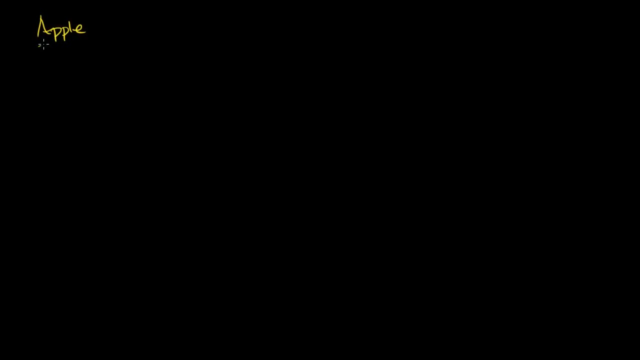 So let's say we are in the apple market. What I want to do in this video is think about both demand and supply for the apples at different prices. So let's draw ourselves a little graph here, And we already know this right over here. 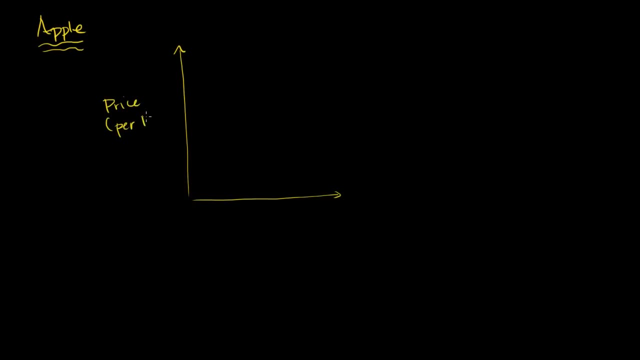 the vertical axis is the price axis And this is we're going to say it's price per pound, And the horizontal axis this is the quantity of apples And let's put some tick marks here. Let's say that's $1 a pound, $2 a pound, $3 a pound, $4 a pound. 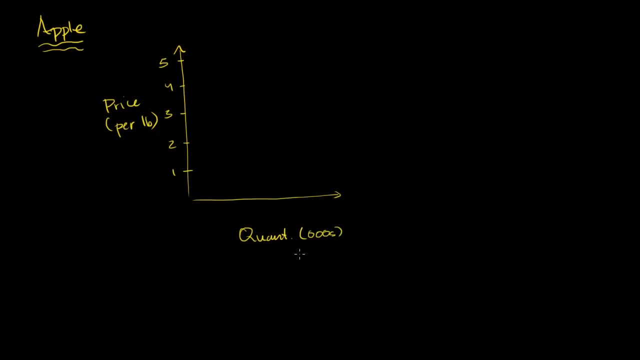 and $5.. And let's say that this is thousands of pounds produced And we have to set a period. So let's say this is all for the next week, And so this is 1,000 pounds, 2,000, 3,000,, 4,000, and 5,000.. 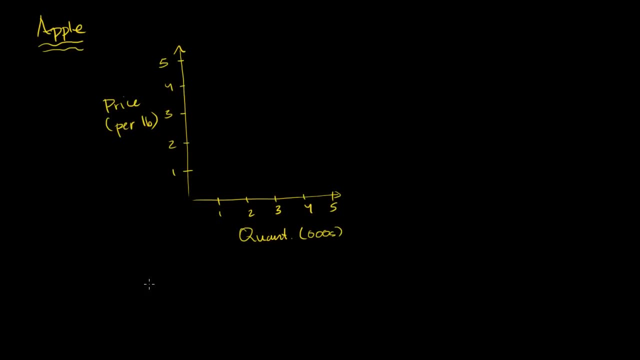 Now let's think about both the supply and the demand curves for this market, or potential supply and demand curves. So first I will do, First I will do the demand. So if the price of apples were really high- and I encourage you to always think about this when you're- 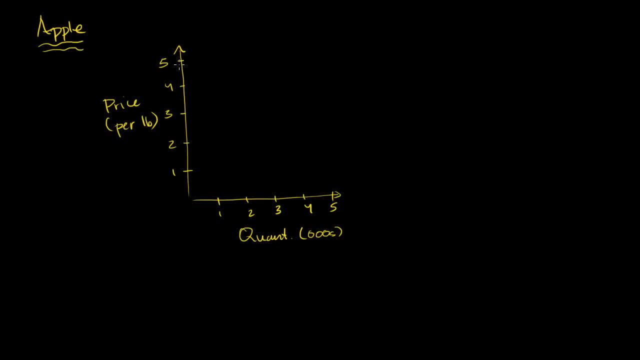 about to draw your demand and supply curves. If the price of apples were really high, what would happen to consumers? Well, they wouldn't demand much, So the quantity demanded would be low. So if the price were high, maybe the quantity demanded 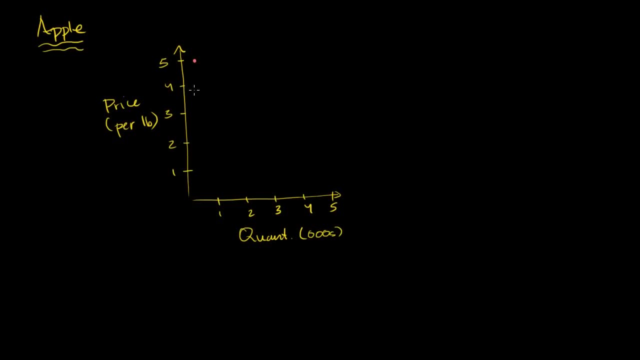 is like 500 apples And once again I'm being very careful to say the quantity demanded is 500 apples. I'm not saying the demand is 500 apples. The demand is the entire relationship, The actual, specific quantity. we call that the quantity demanded. 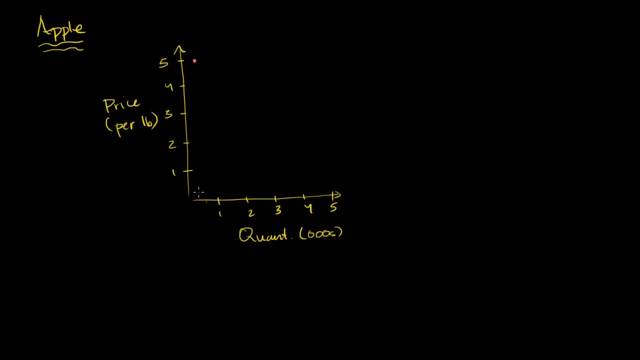 So, at a price of $5, the quantity demanded would be about 500.. Maybe, at a price of $1, the quantity demanded would be maybe 4,000 pounds, And so our demand curve might look something like this: Let me draw it a little bit less bumpy. 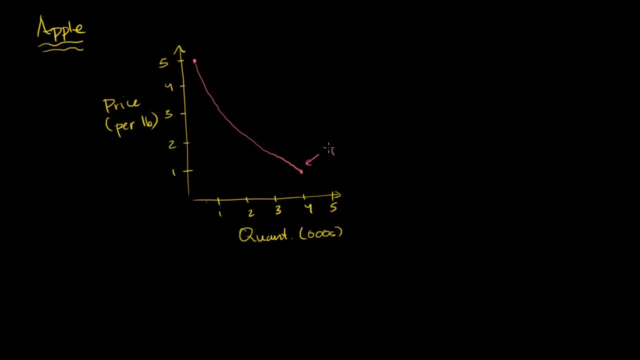 So our demand curve might look something like that. I can label it. That is our demand curve. And now let's think about our supply curve. Well, there's some price below which we aren't even willing to produce apples, So let's say that's like $0.50.. 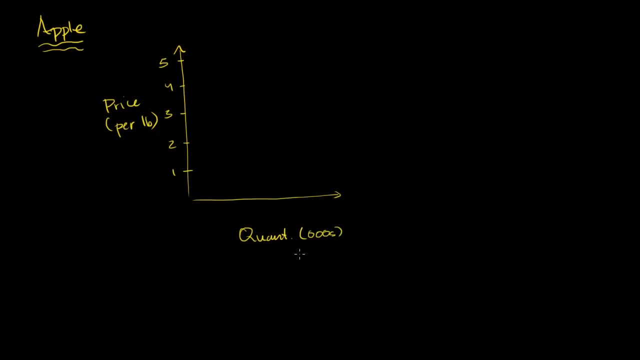 and $5.. And let's say that this is thousands of pounds produced And we have to set a period. So let's say this is all for the next week, And so this is 1,000 pounds, 2,000, 3,000,, 4,000, and 5,000.. 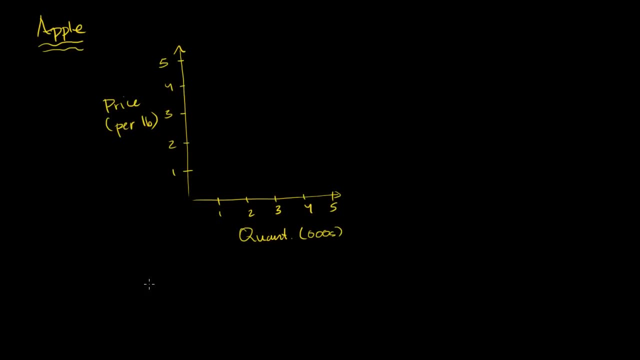 Now let's think about both the supply and the demand curves for this market, or potential supply and demand curves. So first I will do, First I will do the demand. So if the price of apples were really high- and I encourage you to always think about this when you're- 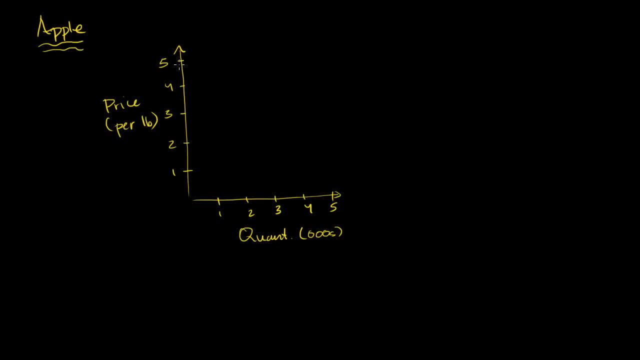 about to draw your demand and supply curves. If the price of apples were really high, what would happen to consumers? Well, they wouldn't demand much, So the quantity demanded would be low. So if the price were high, maybe the quantity demanded 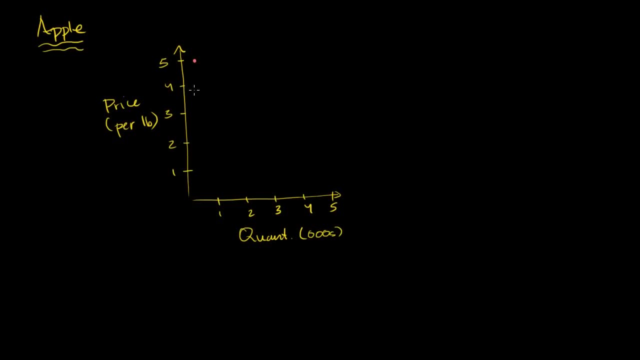 is like 500 apples And once again I'm being very careful to say the quantity demanded is 500 apples. I'm not saying the demand is 500 apples. The demand is the entire relationship, The actual, specific quantity. we call that the quantity demanded. 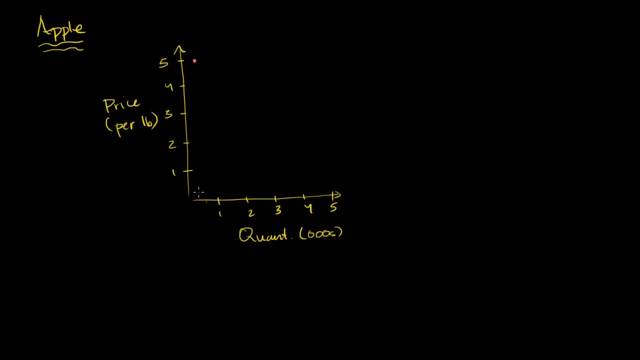 So, at a price of $5, the quantity demanded would be about 500.. Maybe, at a price of $1, the quantity demanded would be maybe 4,000 pounds, And so our demand curve might look something like this: Let me draw it a little bit less bumpy. 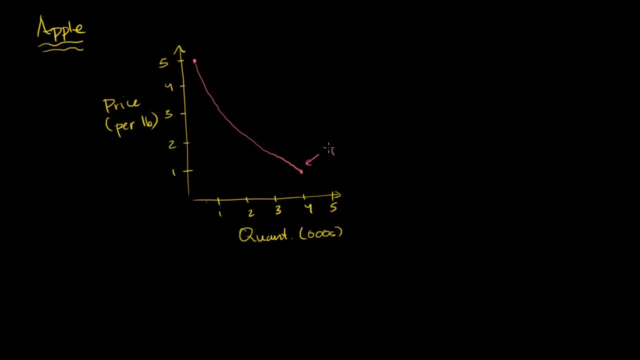 So our demand curve might look something like that. I can label it. That is our demand curve. And now let's think about our supply curve. Well, there's some price below which we aren't even willing to produce apples, So let's say that's like $0.50.. 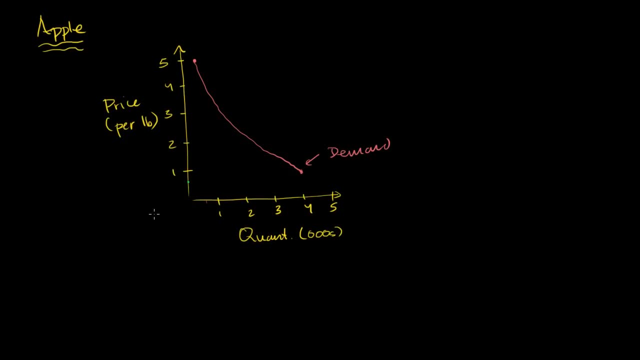 So at $0.50, that's where we're even just willing to start producing apples. Let's say, if the price of apples got to $1, the quantity we'd be willing to supply is about 1,000 pounds. And it just keeps increasing as the price increases. 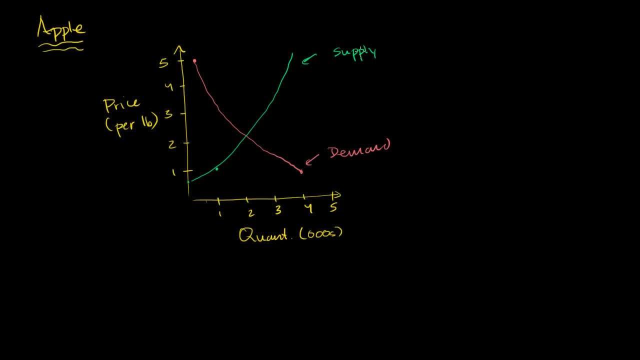 So this is the supply, This is the supply curve, And when I talk about we, I'm talking about all of the suppliers in this market. We could be doing this for a specific supplier. We could be doing this for a specific market. 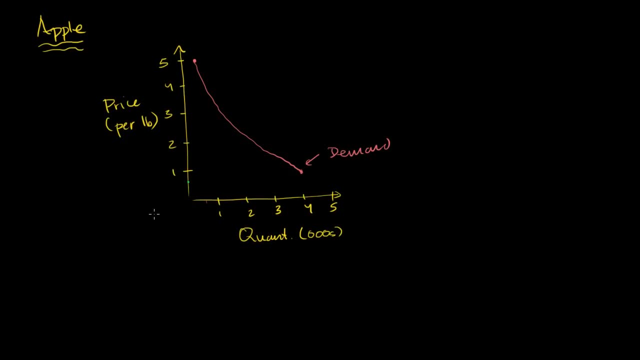 So at $0.50, that's where we're even just willing to start producing apples. Let's say, if the price of apples got to $1, the quantity we'd be willing to supply is about 1,000 pounds. And it just keeps increasing as the price increases. 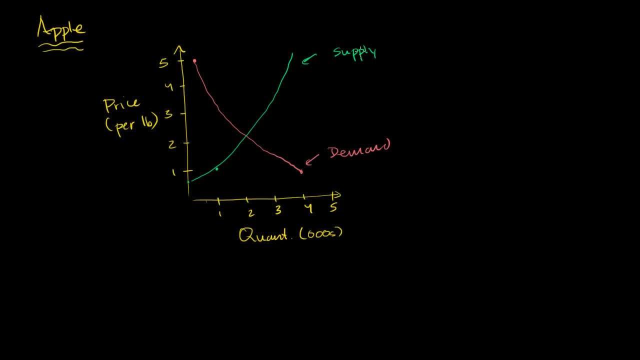 So this is the supply, This is the supply curve, And when I talk about we, I'm talking about all of the suppliers in this market. We could be doing this for a specific supplier. We could be doing this for a specific market. 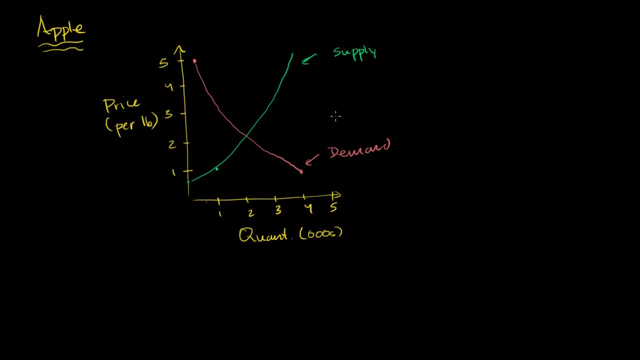 We could be doing this for the global apple market, however you want to view it, But for the sake of this video, let's assume it's like our little town that is fairly isolated and all of that. Now let's think about what happens in different scenarios. 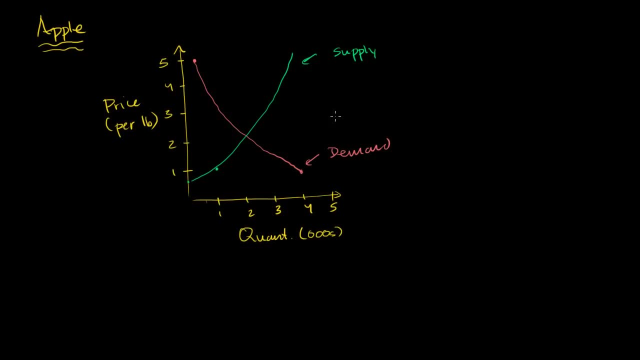 What happens if the suppliers of the apples going into that week for their own planning purposes, they just think, for whatever reason, that they're only going to be able to sell the apples at $1 per pound. And so, given that, given this supply curve, 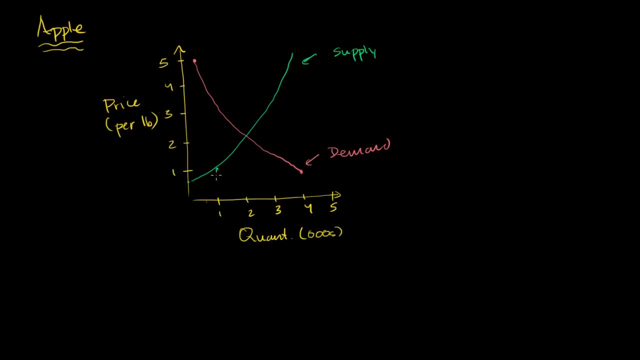 they only supply 1,000 pounds. So this is what the suppliers plan for, And this is where they set the price point at $1 per pound. Now what's going to happen in that scenario? Well, in that scenario, the quantity supplied is 1,000 pounds. 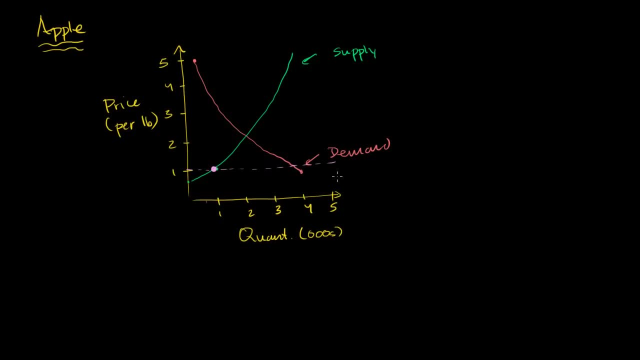 So let me write this down, So I'll do it in pink for this scenario. So in this scenario, the quantity supplied is 1,000 pounds, And what is the quantity demanded? And this is all a scenario where the price or the initial price, 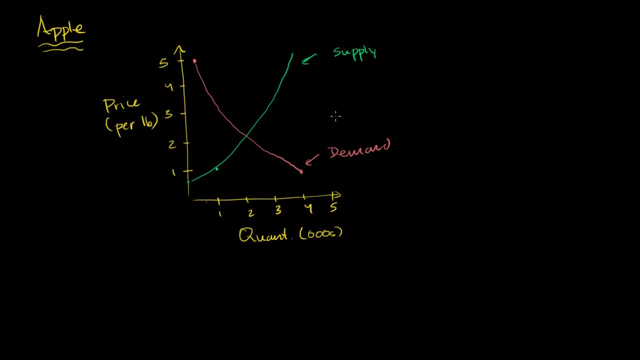 We could be doing this for the global apple market, however you want to view it, But for the sake of this video, let's assume it's like our little town that is fairly isolated and all of that. Now let's think about what happens in different scenarios. 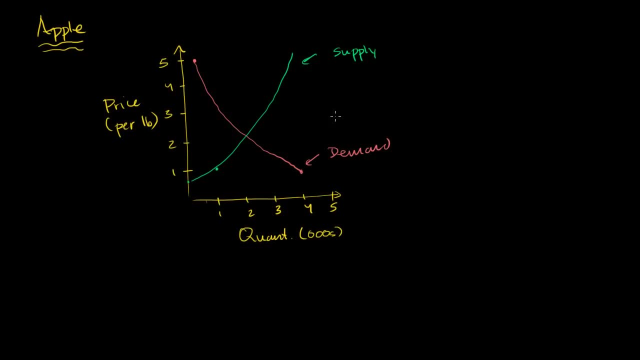 What happens if the suppliers of the apples going into that week for their own planning purposes, they just think, for whatever reason, that they're only going to be able to sell the apples at $1 per pound. And so, given that, given the supply curve, 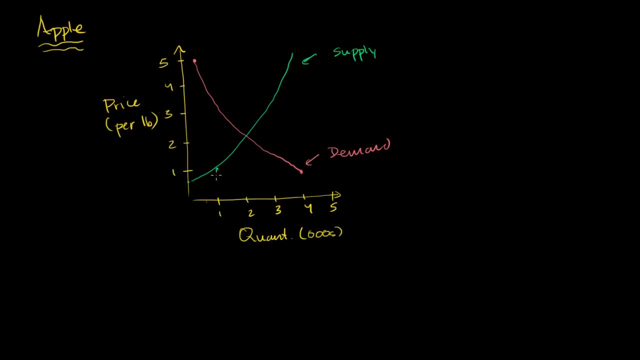 they only supply 1,000 pounds. So this is what the suppliers plan for, And this is where they set the price point at $1 per pound. Now what's going to happen in that scenario? Well, in that scenario, the quantity supplied is 1,000 pounds. 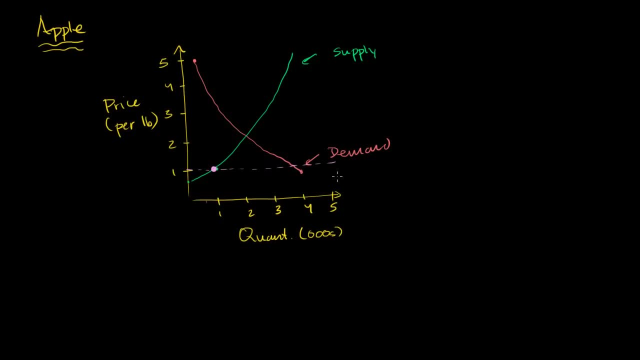 So let me write this down, So I'll do it in pink for this scenario. So in this scenario, the quantity supplied is 1,000 pounds, And what is the quantity demanded? And this is all a scenario where the price or the initial price, 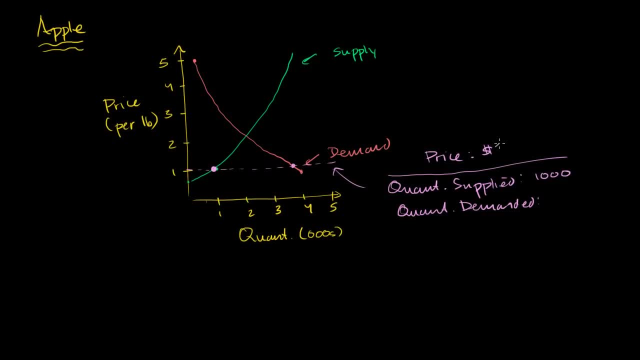 that the growers or the producers set was $1 per pound. $1 per pound, Well, the quantity demanded at $1 per pound is 4,000 pounds of apples. So what do we have here? Well, here we have a shortage. 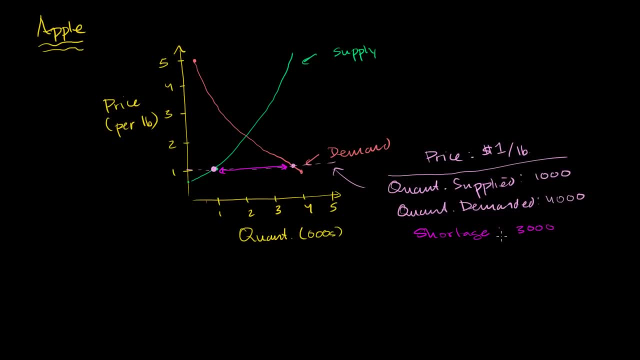 We have a shortage of 3,000 apples. at that price point, At $1,, a lot more people are going to want to buy apples And the producers just didn't. I guess they didn't figure it out. They didn't figure that out right. 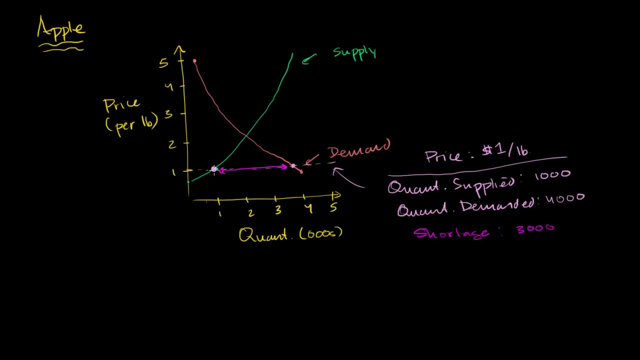 And they didn't produce enough apples. Now, what will naturally start happening? If you have the shortage, you have all these people who want to buy apples and you only have so many apples there. well, what might happen in the next period, in the next week? 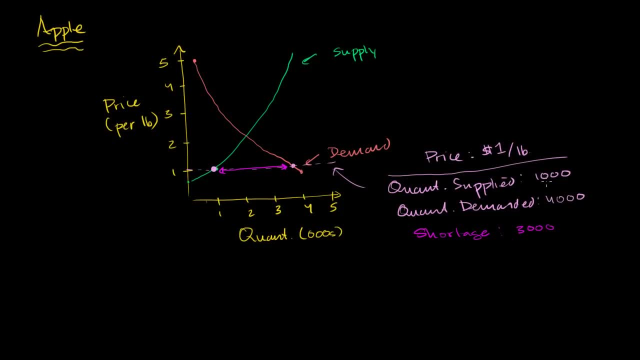 Well, first of all, those apples that are out there. they might get bid up, So the price is going to start going up. The price is going to start going up. People are going to start bidding up the apples. They want them so badly. they're going to start bidding them up. 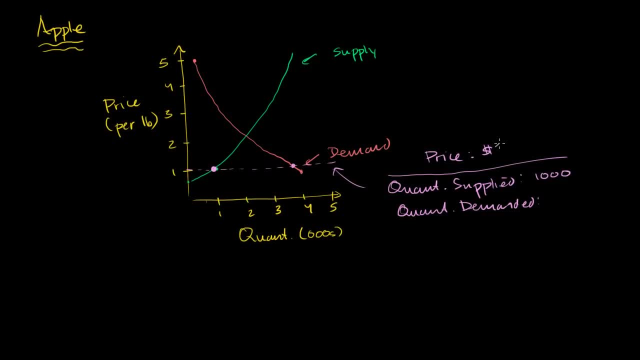 that the growers or the producers set was $1 per pound. $1 per pound, Well, the quantity demanded at $1 per pound is 4,000 pounds of apples. So what do we have here? Well, here we have a shortage. 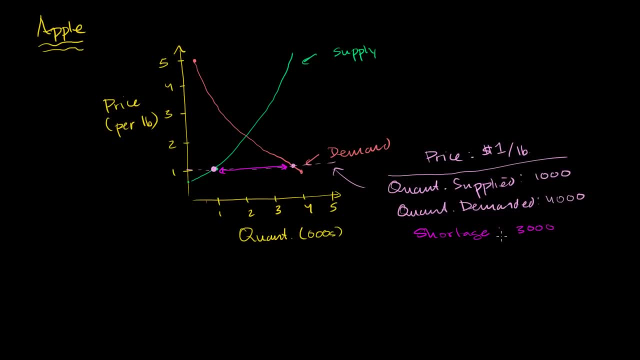 We have a shortage of 3,000 apples. at that price point, At $1,, a lot more people are going to want to buy apples And the producers just didn't. I guess they didn't figure it out. They didn't figure that out right. 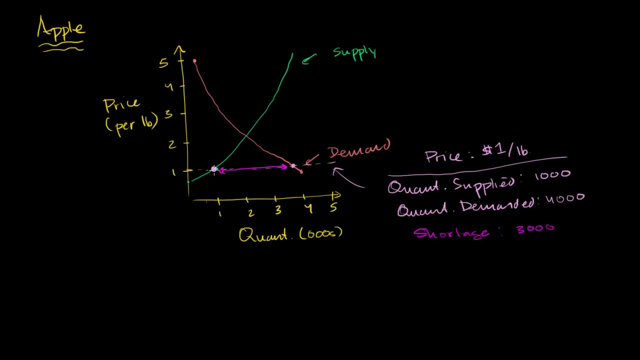 And they didn't produce enough apples. Now, what will naturally start happening? If you have the shortage, you have all these people who want to buy apples and you only have so many apples there. well, what might happen in the next period, in the next week? 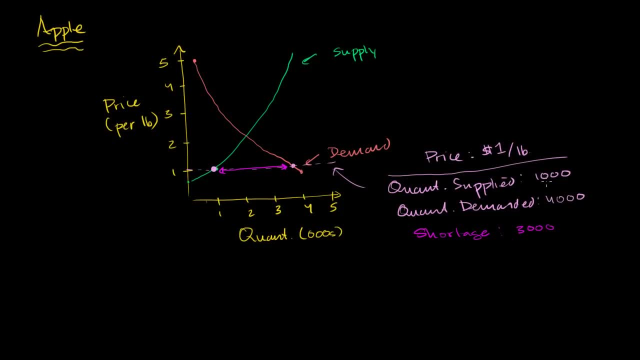 Well, first of all, those apples that are out there. they might get bid up, So the price is going to start going up. The price is going to start going up. People are going to start bidding up the apples. They want them so badly. they're going to start bidding them up. 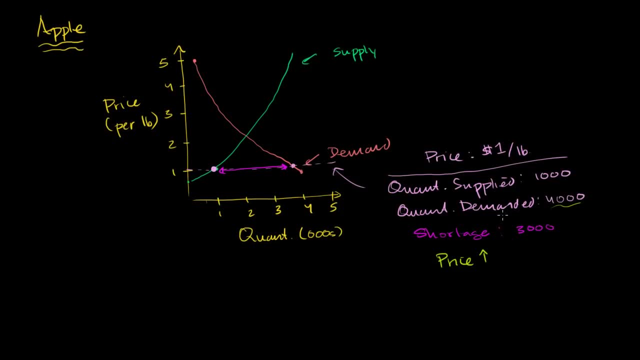 And as they start getting bid up, the producers are going to say: wow, there's so many people, We're running out of apples. We also need to increase the quantity produced, And so the quantity will also go up, So the price will go up. 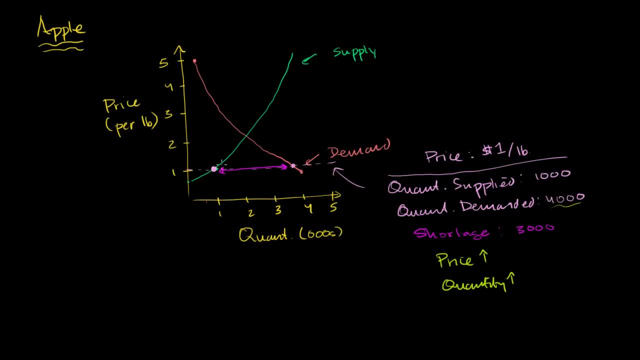 If you look at it from the supplier's point of view, the price will go up and the quantity will go up. They will move along this line there. So maybe in the next period there's less of a shortage Or they move away from that shortage situation. 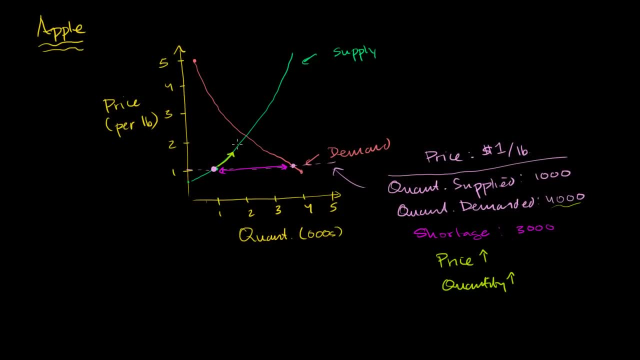 If the price and quantity increase a little bit. so maybe the price goes to $2 and the quantity goes to. I don't know. this looks like about 1,900 pounds. Now, all of a sudden you have less of a shortage. 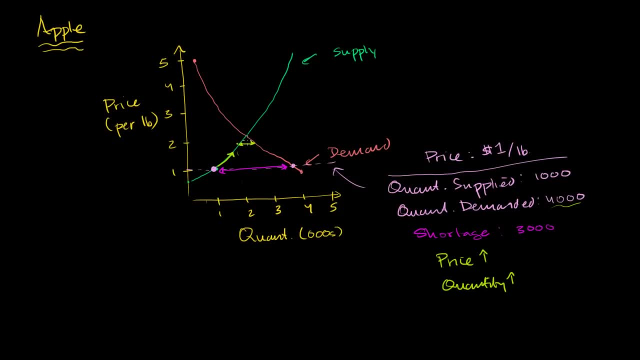 And I think you see that I'm getting to an interesting point over here, But I won't go there just yet. I won't go there just yet. Now let's think about another situation. Let's think about after this happens. price and quantity increases so much. 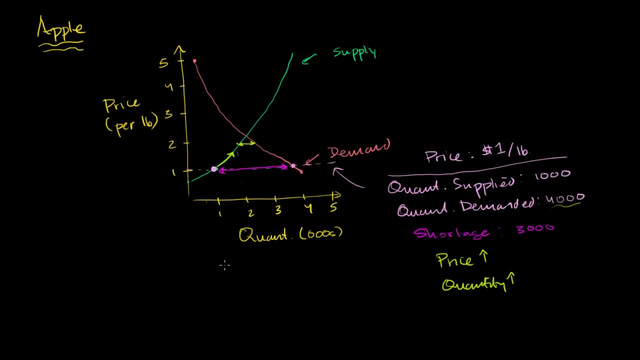 that it essentially overshoots this interesting point right over here. So in the next week the suppliers will say, wow, people want our apples, badly listed, at the price, really high, at $3.. And at $3, we're really excited about producing apples. 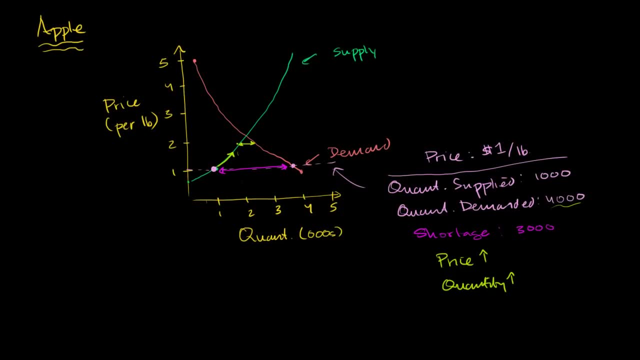 So we, the suppliers, are going to produce- Let me do this in a color I haven't used yet- We, the suppliers, are going to produce at $3 a pound. We're hoping to sell 3,000 pounds of apples. 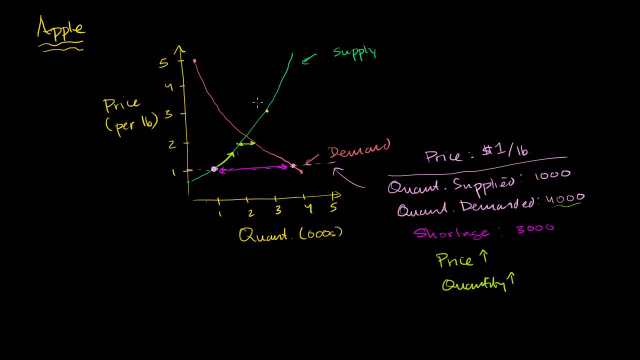 So this is maybe where they adjust to the next week. But what's going to happen there at a price of $3?? So that's this scenario right over here: the price of $3.. So the price is now $3 per pound. 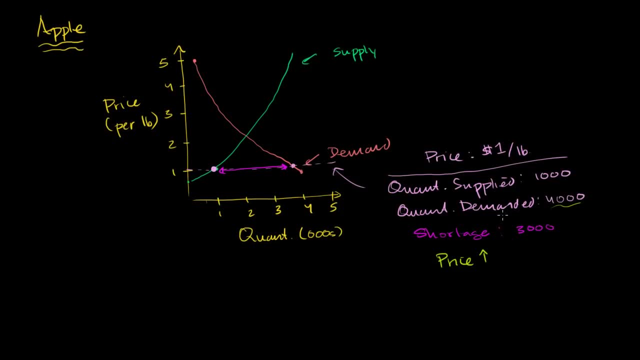 And as they start getting bid up, the producers are going to say: wow, there's so many people, We're running out of apples. We also need to increase the quantity produced, And so the quantity will also go up, So the price will go up. 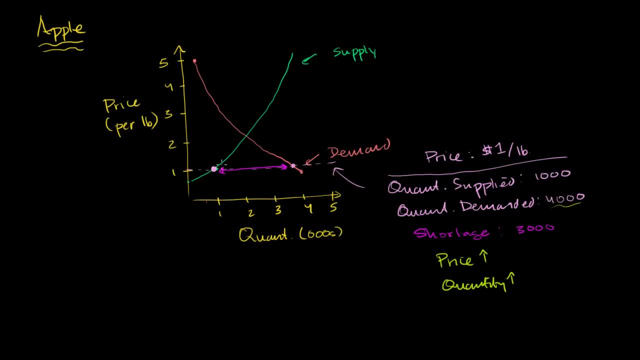 If you look at it from the supplier's point of view, the price will go up and the quantity will go up. They will move along this line there. So maybe in the next period there's less of a shortage Or they move away from that shortage situation. 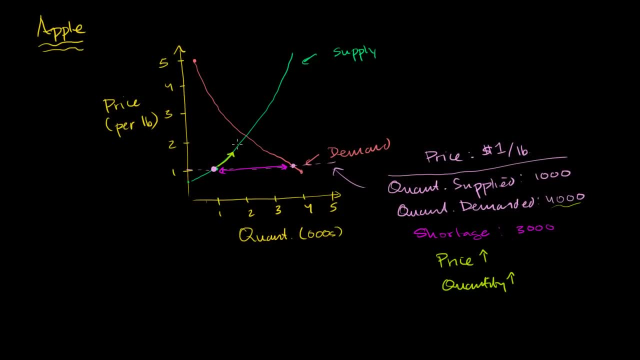 If the price and quantity increase a little bit. so maybe the price goes to $2 and the quantity goes to. I don't know. this looks like about 1,900 pounds. Now, all of a sudden you have less of a shortage. 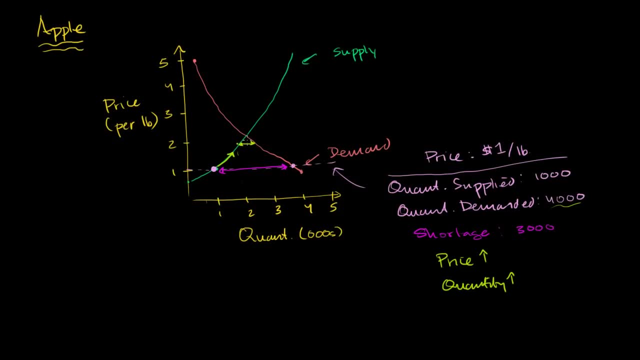 And I think you see that I'm getting to an interesting point over here, But I won't go there just yet. Now let's think about another situation. Let's think about after this happens. price and quantity increases so much that it essentially overshoots this interesting point, right? 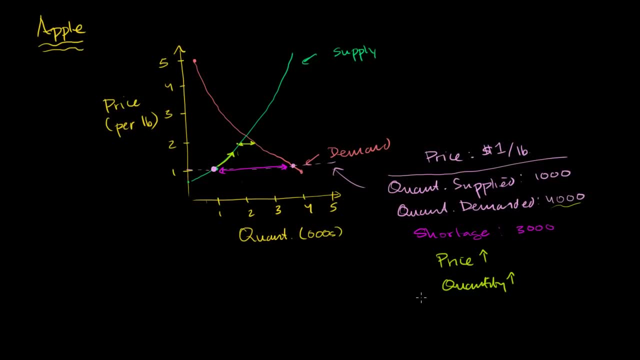 over here. So in the next week the suppliers will say, wow, people want our apples, badly listed at the price, really high, at $3. And at $3, we're really excited about producing apples. So we, the suppliers, are going to produce. 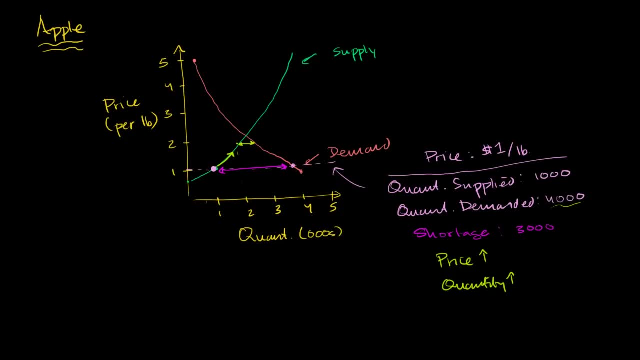 Let me do this in a color I haven't used yet. We, the suppliers, are going to produce at $3 a pound. We're hoping to sell 3,000 pounds of apples, So this is maybe where they adjust to the next week. 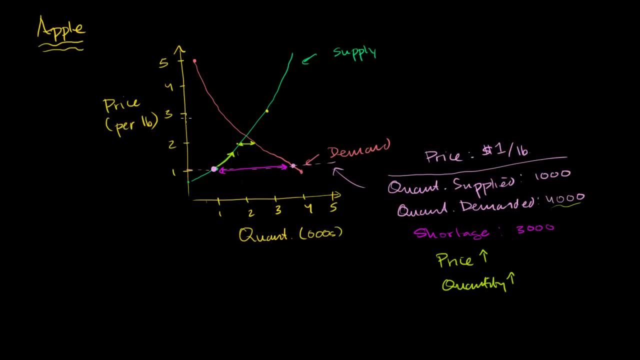 But what's going to happen there at a price of $3?? So that's this scenario right over here: the price of $3.. So the price is now $3 per pound. Well, now the quantity supplied is going to be 3,000 pounds. 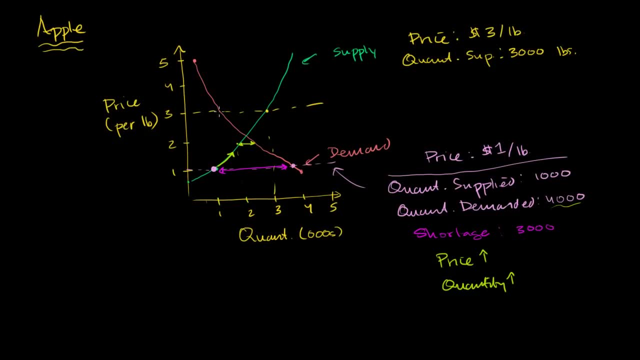 I could write 3,000 pounds. And what is the quantity demanded? The quantity demanded is now Much lower. The price is high now because consumers might want to go buy other things, or they can't afford an apple, or whatever it might be. 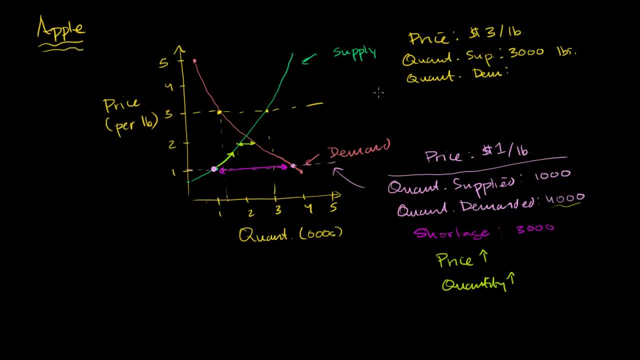 And so now the quantity demanded, that looks like about 1,300 pounds. So what situation do we have now? Well, now we have a much bigger supply, or the quantity supplied is much bigger than the quantity demanded. So now we face a surplus. 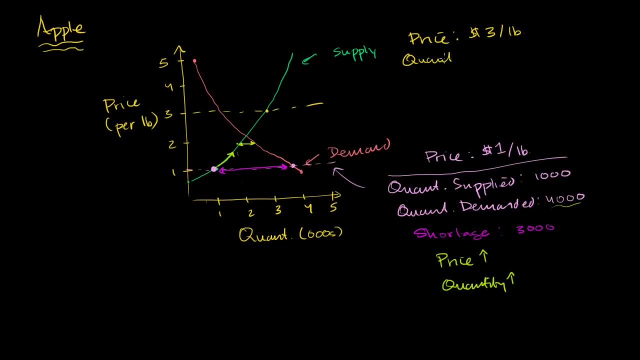 Well, now the quantity supplied is going to be 3,000 pounds. I could write 3,000 pounds, And what is the quantity demanded? The quantity demanded is now Much lower. The price is high now because consumers might want to go buy other things. 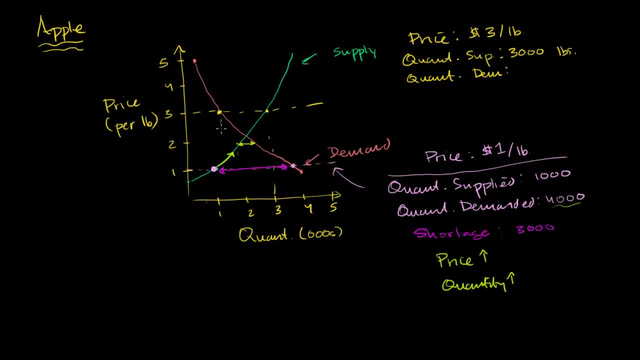 or they can't afford an apple, or whatever it might be, And so now the quantity demanded? that looks like about 1,300 pounds. So what situation do we have now? Well, now we have a much bigger supply. 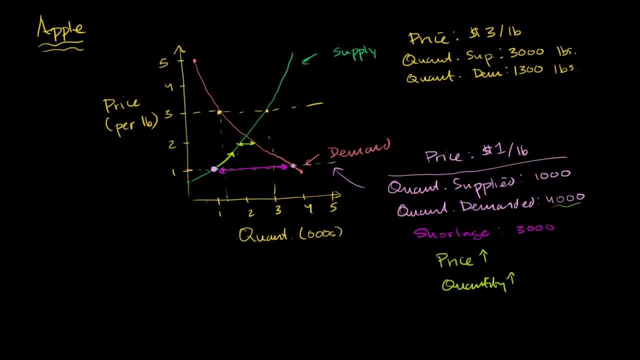 or the quantity supplied is much bigger than the quantity demanded. So now we face a surplus, So now we have a surplus. Actually, let me not draw that line there. I want to make it clear. this is all the same scenario. 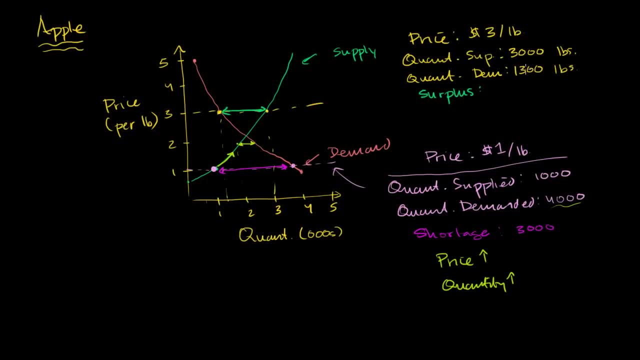 We now have a surplus of what is this? 700 will get us to 2,000.. We have a surplus of 1,700 pounds of apples. And now what happens in a surplus situation? Well, apples won't stay good forever. 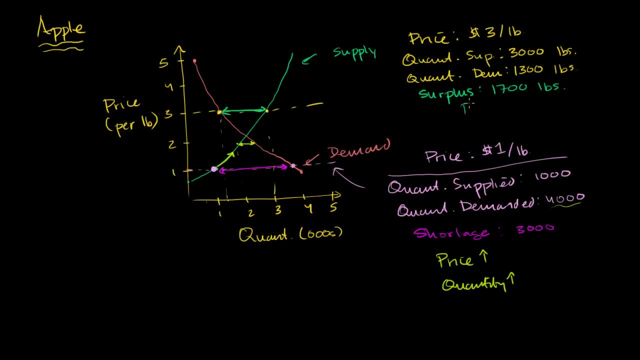 So maybe the producers get a little desperate, So they start selling, They start reducing the price, maybe to start attracting some consumers, So they start reducing the price. And also when they start seeing that the price is going down and you have this glut of apples and that they're all going bad, 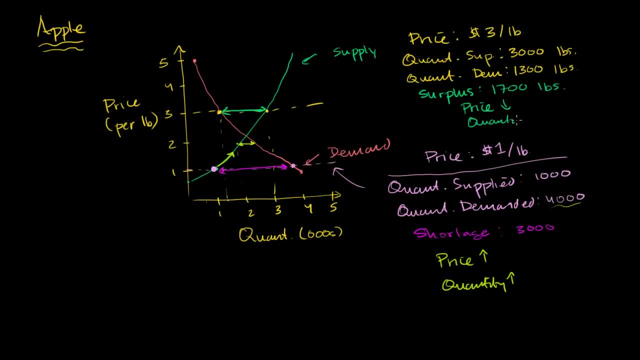 and they're not getting sold. the quantity is also going to start going down. They'll produce fewer and fewer apples, And so we'll move here along the supply curve. And as you decrease the price, what's going to happen to the demand curve? 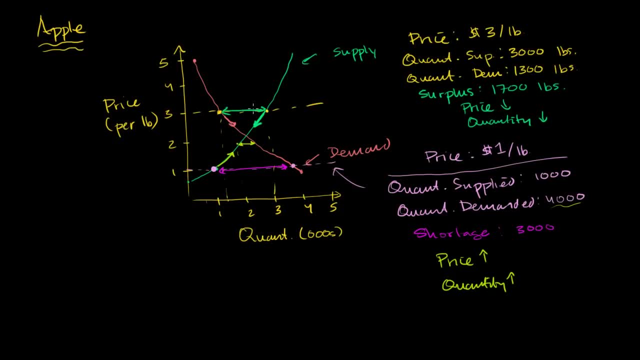 Well, the demand is going to go up. So over here the price was too high, So it's natural for the sellers to lower the price, And so when you lower the price, it also reduces the quantity. We go this way. And when you lower the price it increases demand. You go that way. If the price from the get-go were too low, then you have this huge shortage. Things get bid up, The prices go up. As the price goes up, the suppliers. 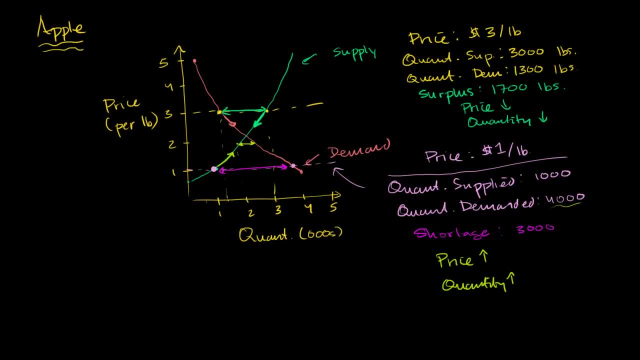 want to produce more, They move up the curve And as the price goes up, then the people will demand less. And you see that it's all converging on a point right over here Where the two lines intersect, And let me do that in a. it's all converging right over there. 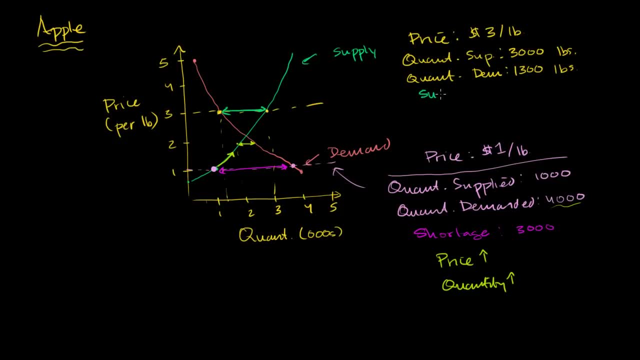 Actually, let me not draw that line there. I want to make it clear. this is all the same scenario. We now have a surplus of what is this? 700 will get us to 2,000.. We have a surplus of 1,700 pounds of apples. 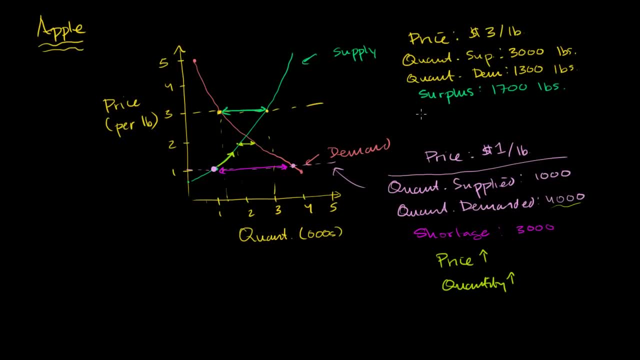 And now what happens in a surplus situation? Well, apples won't stay good forever, So maybe the producers get a little desperate, So they start selling. They start reducing the price, maybe to start attracting some consumers, So they start reducing the price. 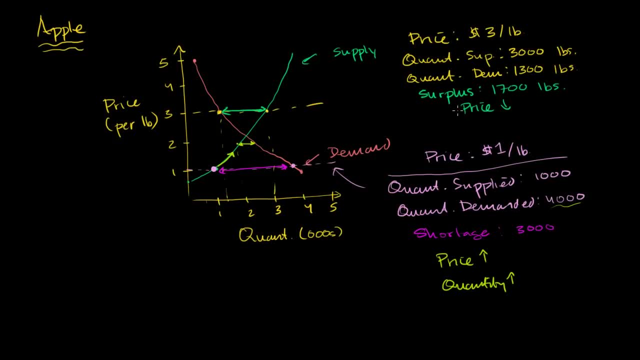 And also when they start seeing that the price is going down and you have this glut of apples and that they're all going bad and they're not getting sold, the quantity is also going to start going down. They'll produce fewer and fewer apples. 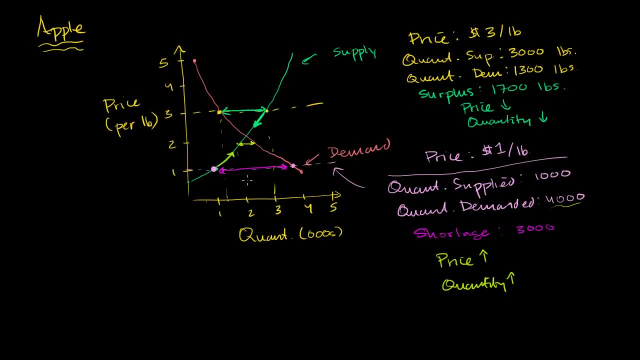 And so we'll move here along the supply curve. And as you decrease the price, what's going to happen to the demand curve? Well, the demand is going to go up. So over here the price was too high, So there's a demand. 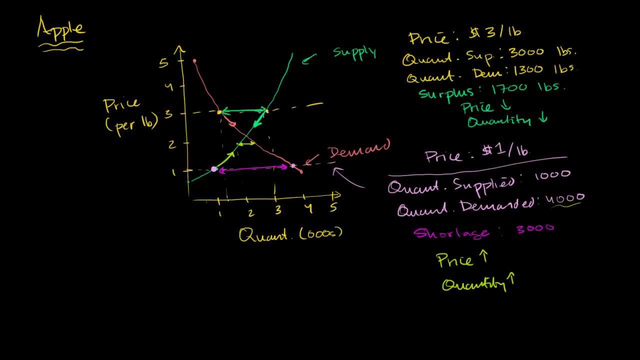 It's natural for the sellers to lower the price, And so when you lower the price, it also reduces the quantity. We go this way, And when you lower the price, it increases demand. You go that way If the price from the get-go were too low. 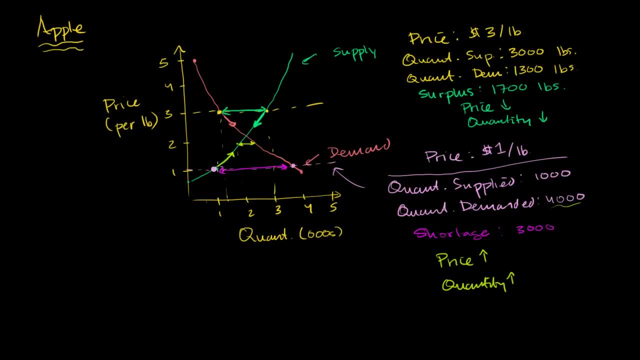 then you have this huge shortage. Things get bid up, The prices go up. As the price goes up, the suppliers want to produce more, They move up the curve, And as the price goes up, then the people will demand less. And you see that it's all converging on a point. 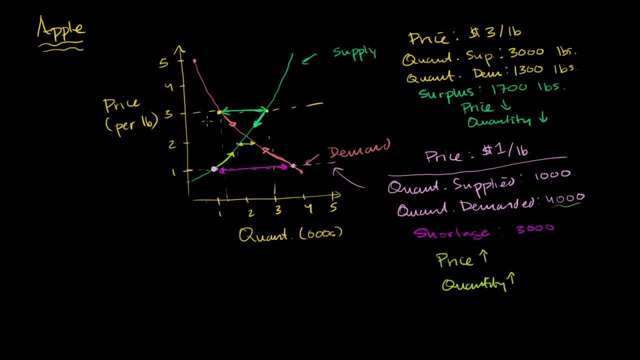 right over here where the two lines intersect, And let me do that in a. it's all converging right over there And that's the point at which supply, that's the price at which this is the price at which the quantity supplied. 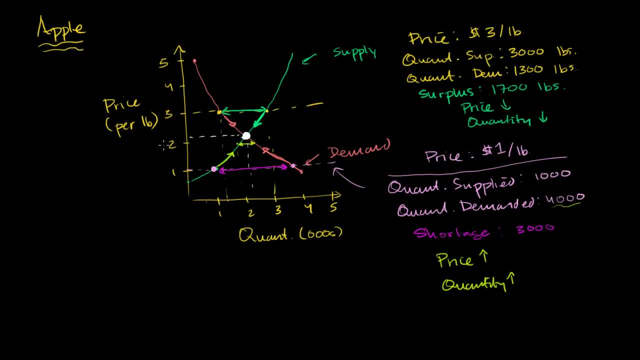 will equal the quantity demanded And we call this price, we call this, which looks like for this scenario, maybe about $2.15.. So let me just write it there. So $2.15, we call that the equilibrium price. 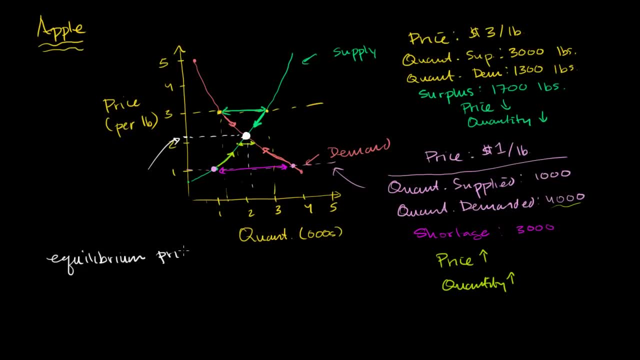 Equilibrium. Equilibrium price is $2.15 a pound, And it's the price at which the quantity supplied is equal to the quantity demanded. And so this quantity, where the quantity supplied is equal to the quantity demanded, that's the equilibrium quantity. 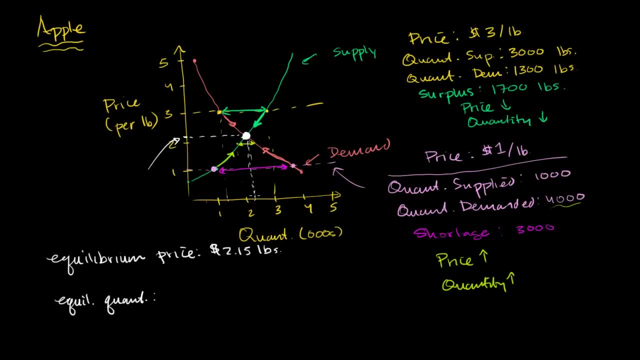 And that right over here looks like it's right about- I don't know- 2,200 pounds And, assuming nothing else changes, this is a good scenario for both the consumers and the producers. They keep producing 2,200.. They charge this price. 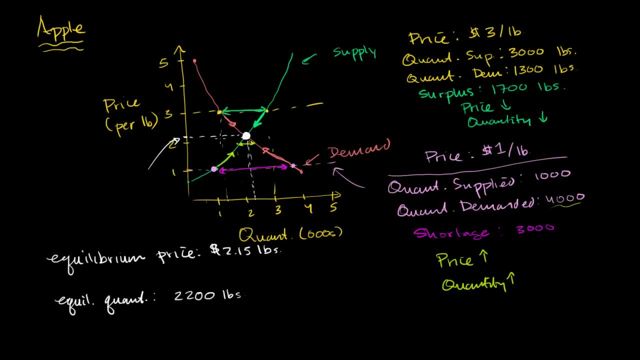 And everything's happy. All the apples get sold and none of them go bad. 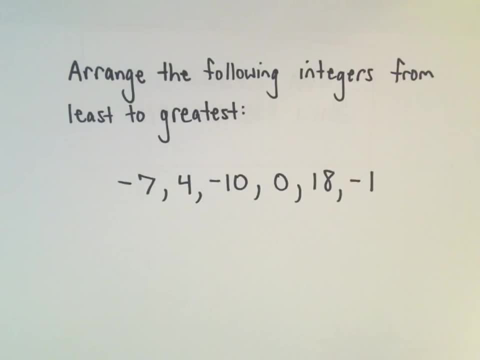 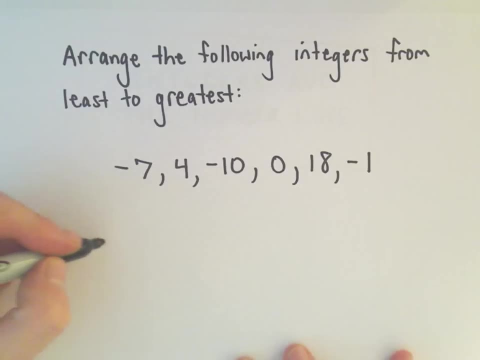 Alright, in this example we're going to arrange some integers from the least to the greatest. We've got negative 7, positive 4, negative 10, 0, 18, and negative 1.. And again, maybe it's easiest to think about a number line. 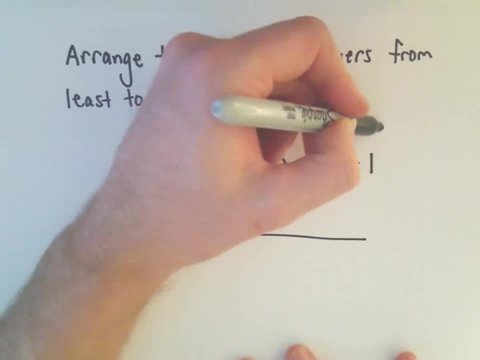 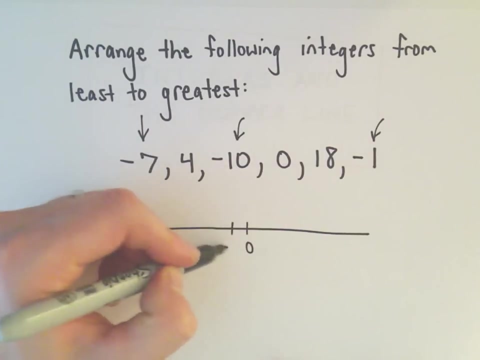 So the first thing I do is pick out my negative values, So I know those are going to be the smallest numbers. Well, let's see if there's 0, negative 1 would be right about there. I'm not going to fill in every digit. 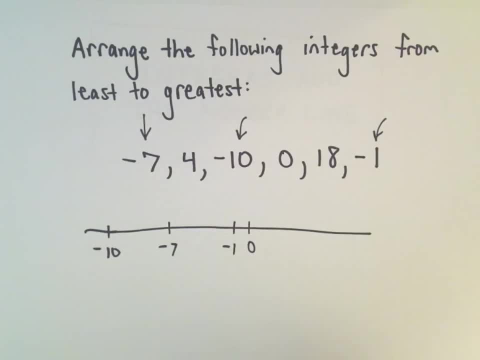 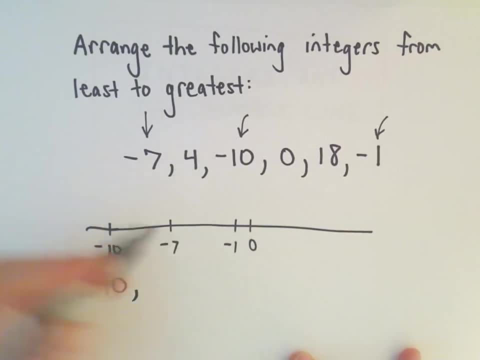 But there's negative 7. And negative 10 would be the furthest one to the left. So that means negative 10 would be our smallest number. Let's see, I guess the next one would be negative 7.. And then we would have negative 1.. 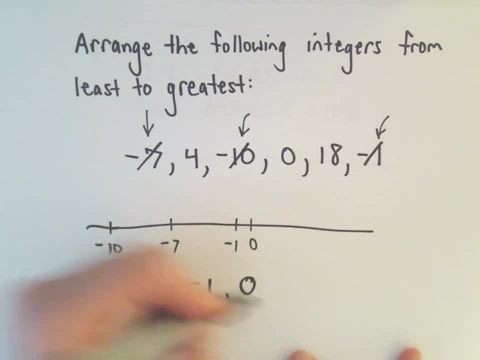 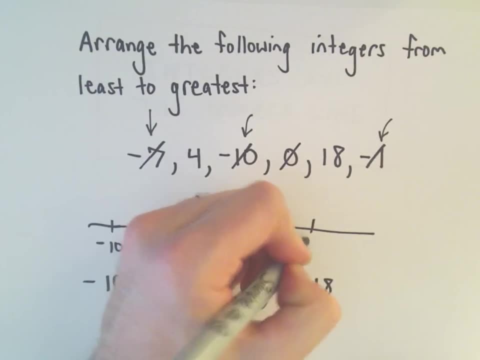 So that takes care of those. 0 would be the next number. And then, last but not least, we've got 4 and 18.. Well, certainly 4 is smaller than 18.. And now we've got our numbers arranged from least to greatest. predictions from year one. So the next one is negative 6. It's smaller than the last one. And then case number number three. Let's see here at 5. The first time we did, it is negative 8.. Our number one will be a condition.